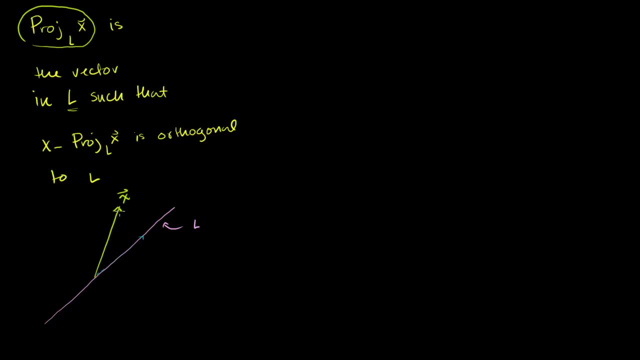 to everything in L. It's going to be orthogonal to everything in L, Just like that. So this right here would be its difference vector, That would be x minus the projection of x onto L, And then of course, this vector right here. this is the. 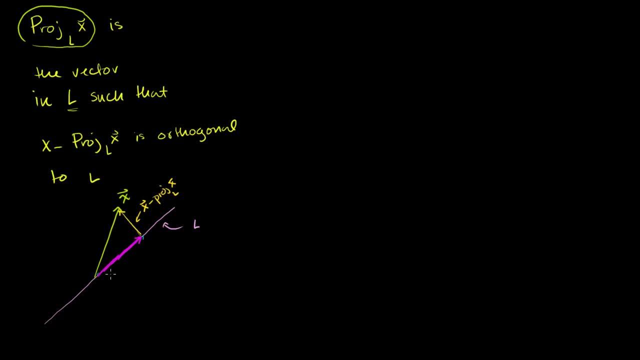 one. we were defining it, That was the projection: Projection onto L of x. Now, what's a different way that we could have written this? We could have written this exact same definition. We could have said: it is the vector in L, such that so we 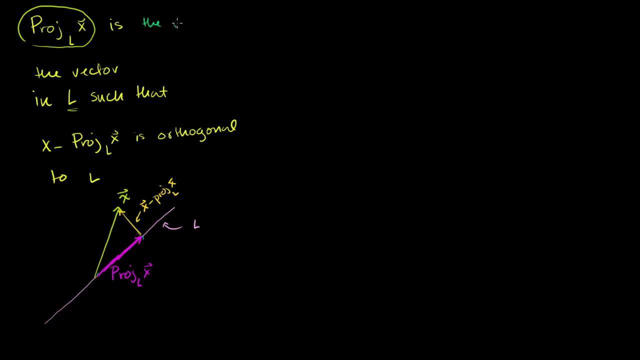 could say: let me write it here in purple: This is the vector v in L, such that v. let me write it this way, such that x minus v, x minus the projection of L is orthogonal. let me write it is equal to w, which is: 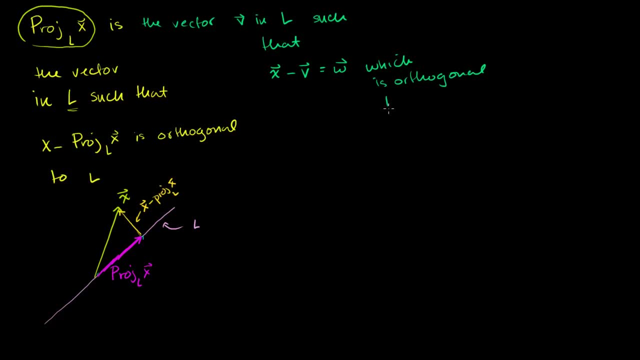 orthogonal to x, It's equal to everything in L. Being orthogonal to L literally means being orthogonal to every vector in L, So I just rewrote it a little bit different. Instead of just leaving it as a projection of x onto L I. 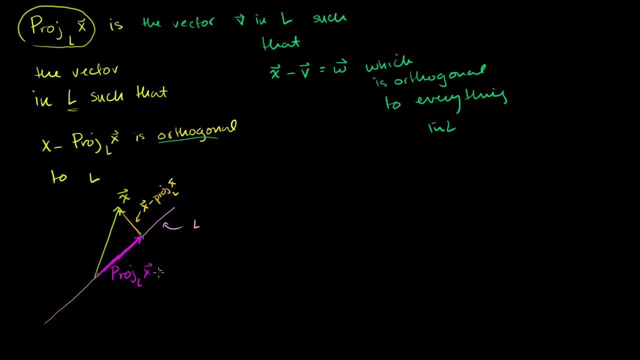 said: hey, that's some vector v in L. So this is some vector v in L, such that x minus v is equal to some other vector w. That's that other vector w which is orthogonal to everything in L, Or we could rewrite that statement right there as x is. 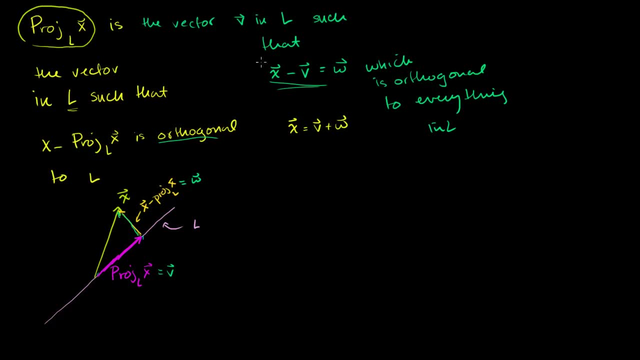 equal to v plus w. So we could just say that the projection of x onto L is the unique vector v in L, such that x is equal to v plus w, where w is a unique vector. I mean it is going to be a unique. 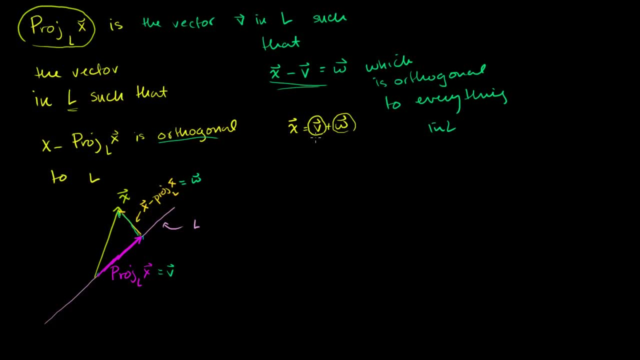 vector in the orthogonal complement of L Right. This has got to be orthogonal to everything in L, So that's going to be a member of the orthogonal complement. It's going to be a member of the orthogonal complement of L, So this definition is actually completely consistent with our. 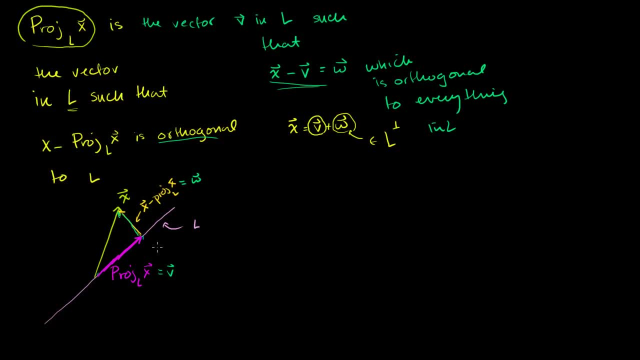 new subspace definition And we could just extend it to arbitrary subspaces, not just lines. And let me help you visualize that. Let's say we're dealing with R3 here And I've got some subspace in R3. And let's say that subspace happens to be a plane. 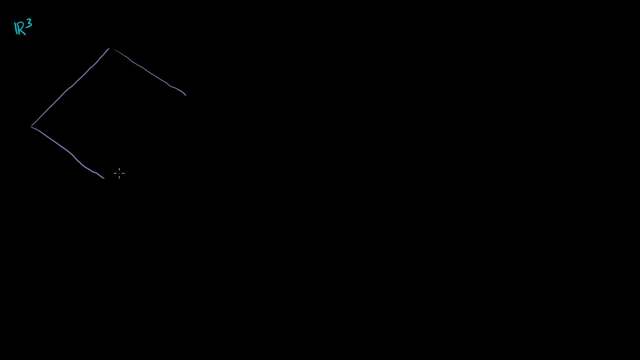 I'm going to make it a plane, just so that it becomes clear that we don't have to take projections just onto lines. So this is my subspace v, right there, And let me draw its orthogonal complement. Let's say its orthogonal complement looks something. 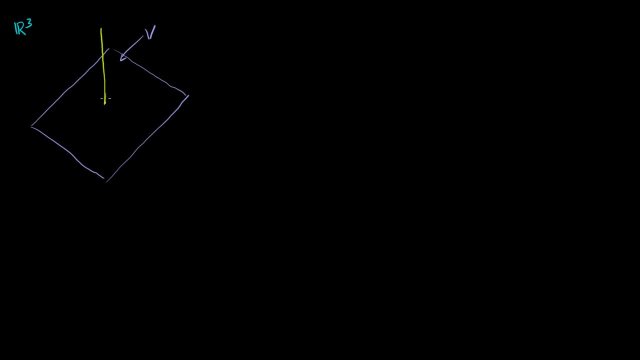 like that. Let's say it's a line And then it intersects right there and then it goes back And of course it would have to intersect at the zero vector Right. OK, Zero vector. That's the only place where a subspace and its orthogonal 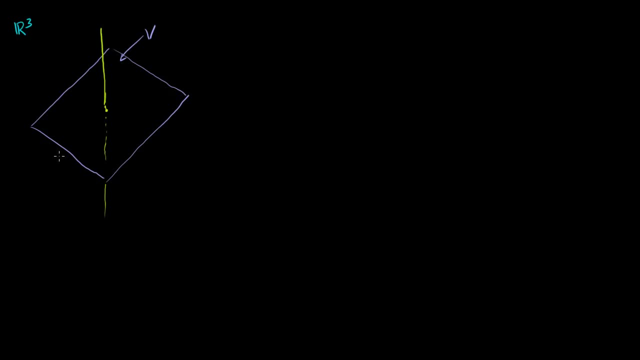 complement, overlap, And then it goes behind and then you can see it again. But obviously you wouldn't be able to see it again because this plane would extend in every direction. But you get the idea. So this right here is the orthogonal. 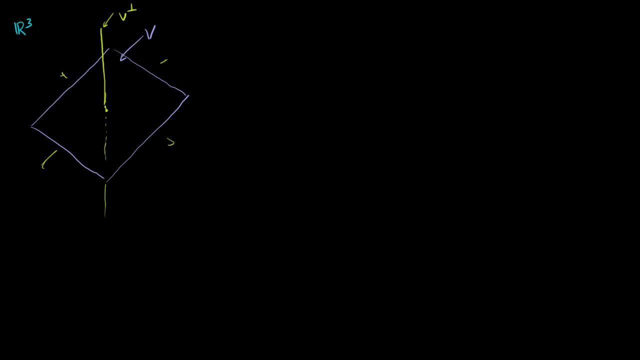 complement of v, That line. Now let's say I have some other arbitrary vector in R3 here. So let's say I have some vector that looks like that. Let's say that that is x. Now our new definition for the projection of x onto v is equal. 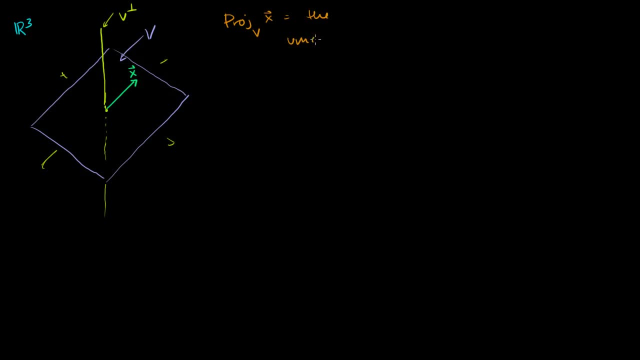 to the unique vector v. This is a vector v That's a subspace v, The unique vector v that is a member of v, such that x is a single vector. So x is equal to v plus w, where w is a unique member of. 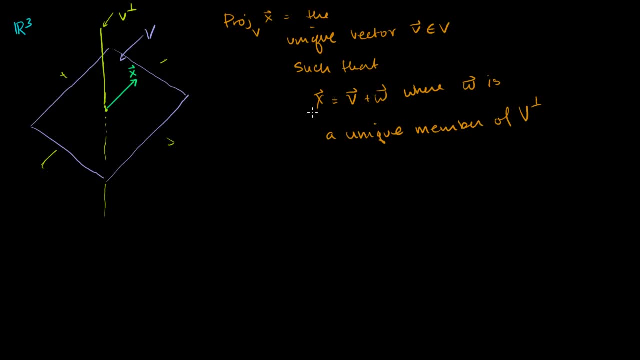 the orthogonal complement of v. This is our new definition. So if we say x is equal to some member of v and some member of its orthogonal complement, we can visually understand that here We could say: OK, It's going to be equal to x. 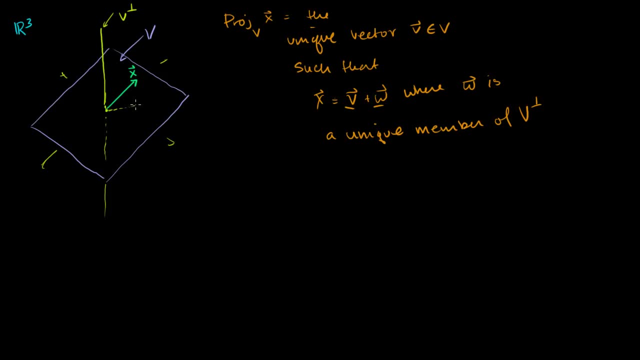 It's going to be equal to. let's see on v, it'll be equal to that vector right there. And then on v's orthogonal complement, you add that to it. So if you were to shift it over, you would get that. 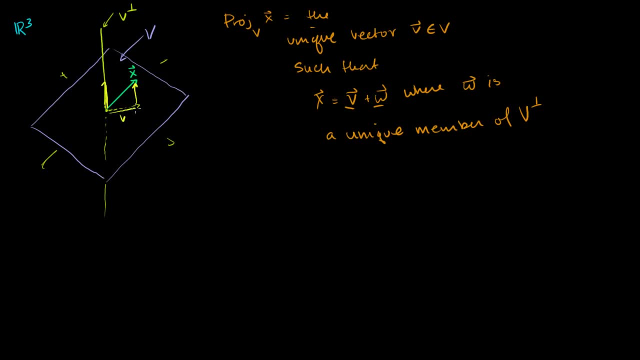 vector just like that. This right here is v, That right there is v. And then this vector that goes up like this out of the plane, orthogonal to the plane is w, And you can see: if you take v plus w, you're going to get x. 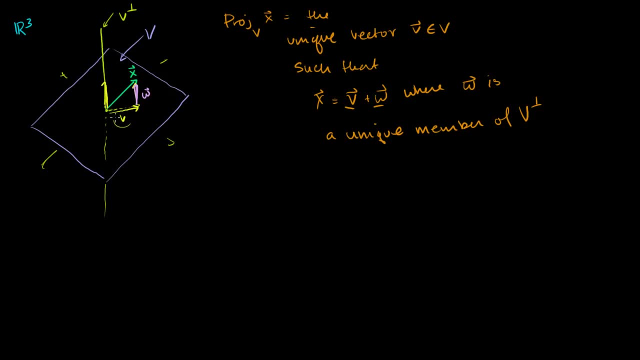 And you can see that v is the projection, The projection onto the subspace capital V. so this is a vector. v is the projection onto the subspace capital V of the vector x. So the analogy to a shadow still holds, If you imagine kind of a light source coming straight down. 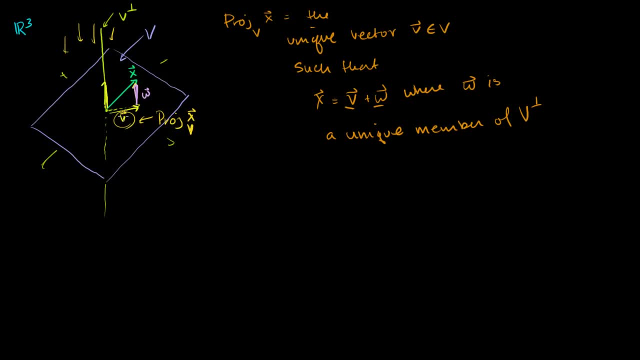 onto our subspace, kind of orthogonal to our subspace. the projection onto our subspace is kind of the shadow of our vector x, So hopefully that helps you visualize it a little bit better. But what we're doing here is we're going to generalize it. 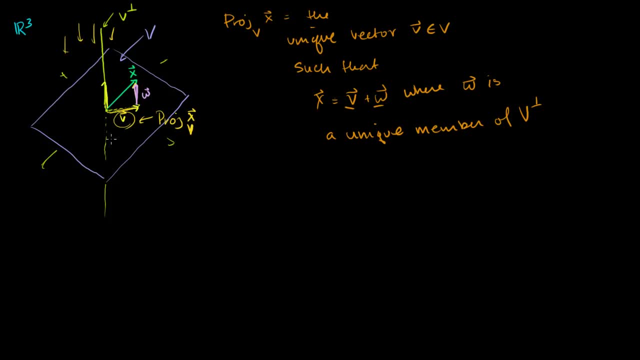 Here I, you know we're going to generalize it. You know, earlier in this video I showed you a line. This is a plane, But we can generalize it to any subspace. This is an r3.. We could generalize it to rn, to r100.. 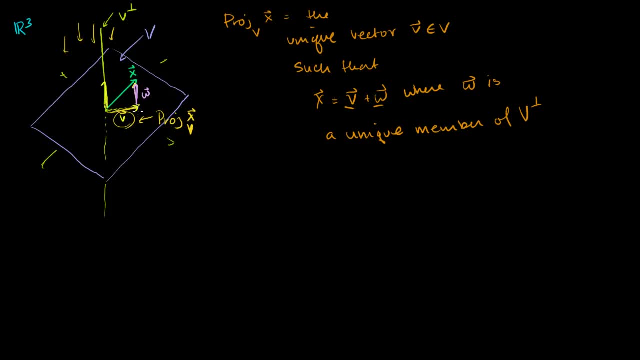 And that's really the power of what we're doing here. It's easy to visualize it here, but it's not so easy to visualize it once you get to higher dimensions. Actually, one other thing: Let me show you that this new definition is pretty much. 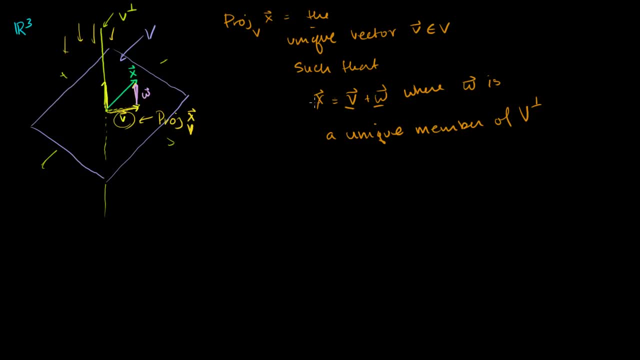 almost identical to exactly what we did with lines. This is identical to saying that the projection onto the subspace x Is equal to some unique vector in v, such that x minus the projection onto v of x is orthogonal. Is orthogonal to x. Is orthogonal to x. 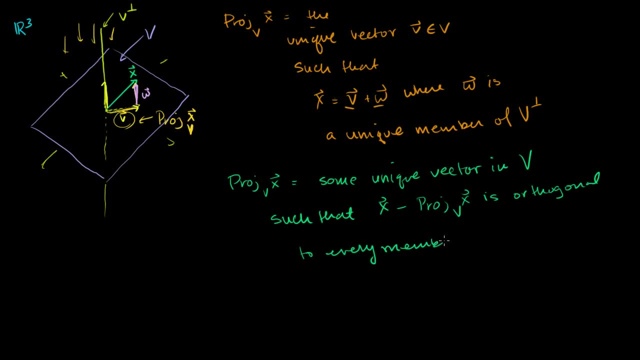 Is orthogonal to x Is orthogonal to every member of v, Because this statement right here is saying: any vector that's orthogonal to any member of v says that it's a member of the orthogonal complement of v. So that statement could be written as x minus the.